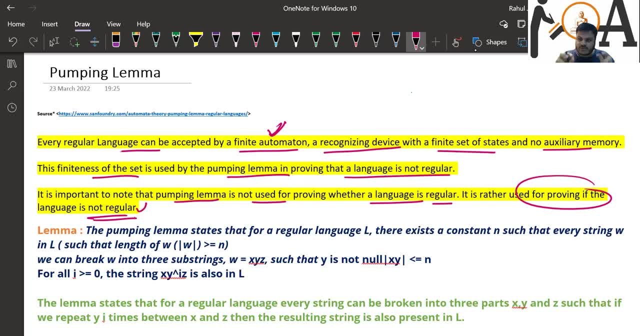 prove whether a language is non-regular, Just to prove non-regular. as a non-regular, we use it. We don't use it in reverse. You can't use this lemma to prove any language is regular. No, You only use it in order to prove that it is non-regular. So one concept. this should: 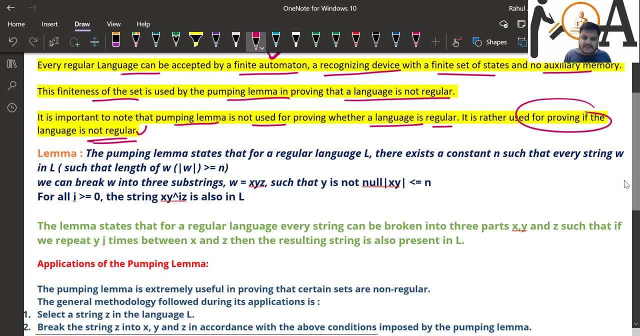 be clear to you Now what lemma exactly says. what lemma exactly says. the pumping lemma states that for a regular language, l, there exists a constant n, such that every string w in l, such that the length of w is greater than or equals to n. We can break w into three. 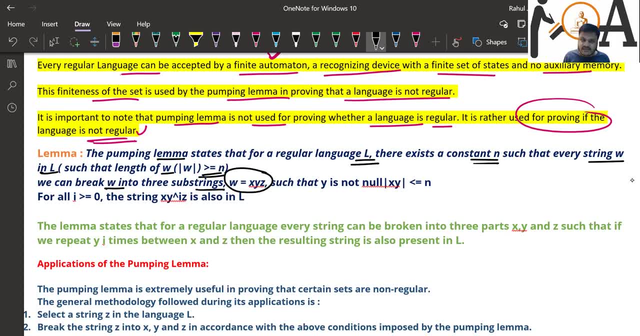 sub strings w equals to x, y, z. We are breaking the sub. we are breaking the string w into three sub strings: x, y and z, such that y is not null. This y is not null, And x and y should be less than or equals to n, For all i greater. 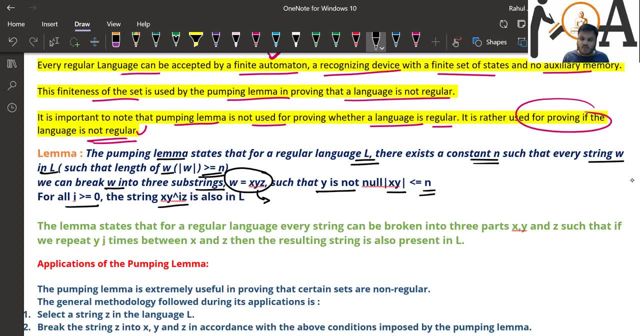 than or equals to 0. the string x, y to the power, i and z is also in l. The lemma states that for a regular language every string can be broken into three parts: x, y and z, such that if we repeat y, 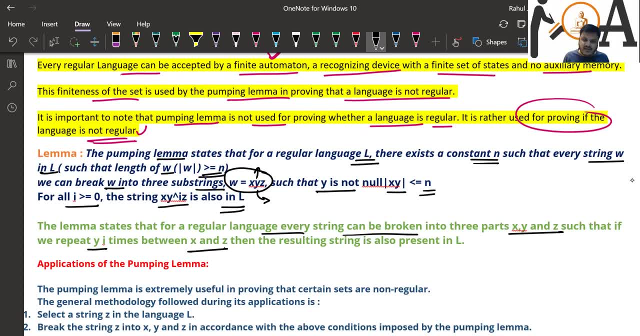 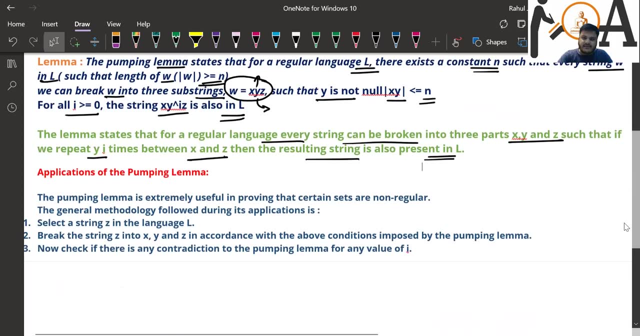 If we repeat this y i times between x and z, then the resulting string is also present in l. If the resulting string is not present in l, it means that it is non-regular. Don't worry, we will take an example and we will let you know that how to solve it. But 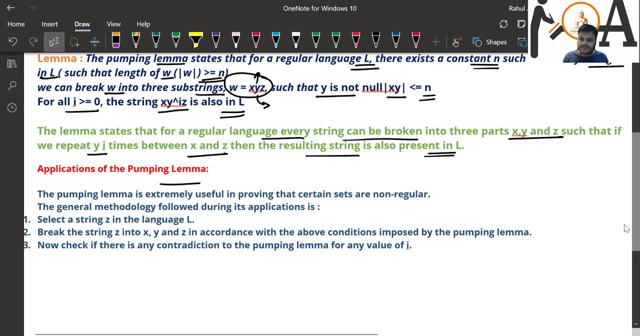 before that, just focus on the applications of the pumping lemma. The pumping lemma is extremely useful in proving that certain sets are non-regular, For example, the general methodology followed during its application is: select a string z in the language l, Break the string z into x, y and z in accordance with the above conditions imposed. 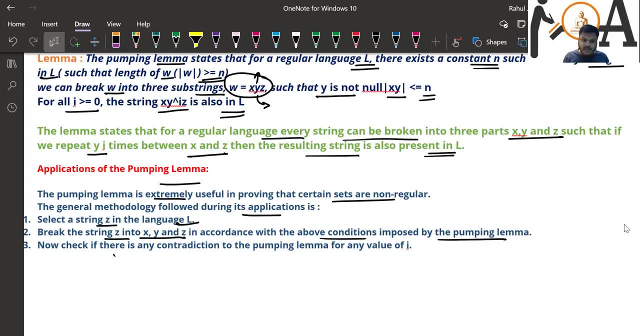 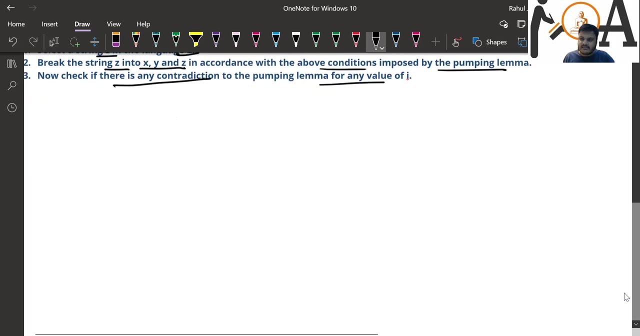 by the pumping lemma And now check if there is any contradiction for the pumping lemma or not for any value of i. If there is a contradiction, it means that it is non-regular. Ok, So basically, pumping lemma is contradiction based algorithm to prove any non-regular language is a non-regular. 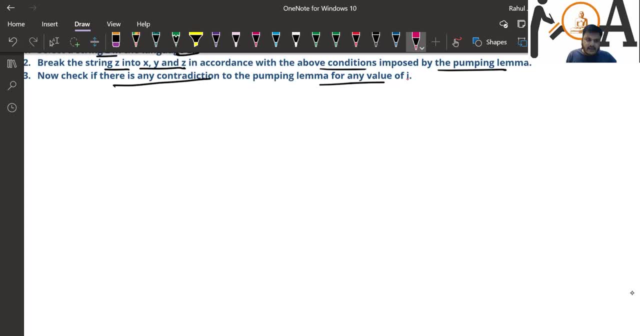 Now let's take an example. Let's say there is a language, l equals to a to the power n and b to the power n where, let's say, n is greater than or equals to 1. We have to prove that this is non-regular, that this is non-regular. So how to implement this pumping lemma? First, 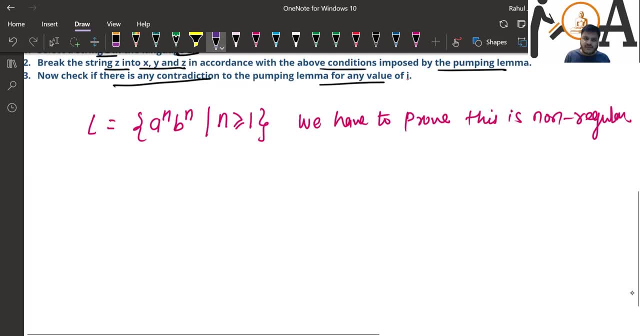 just go contradict. If we have to prove that it is a non-regular, then step 1: assume l is a regular. assume L is regular language. Okay Now, if L is regular language, it means that there is a certain finite set of states on which this language will be accepted, isn't it? 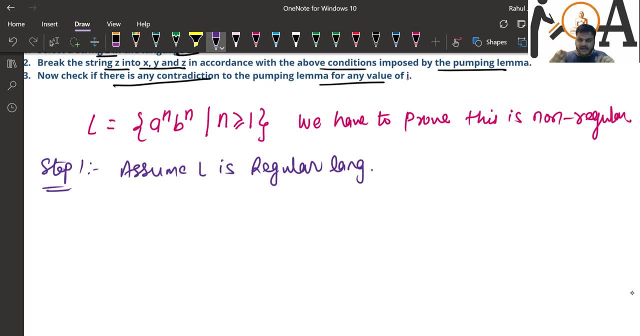 Because if it is a regular, language means regular expression is possible. If regular expression is possible, it means that finite state of finite sets are possible, of finite state sets are possible in which this language will be accepted, then we can say that it is a regular. So if it is a regular, it means that finite automata is possible, And then 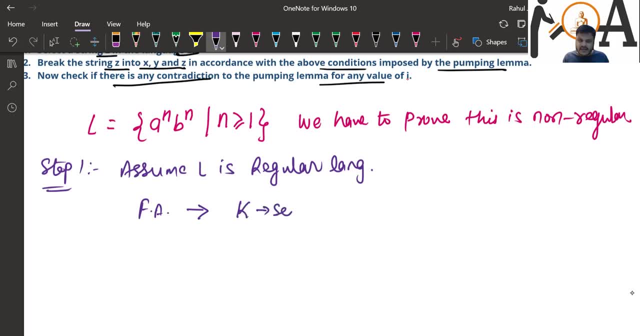 that finite automata may consist finite sets, let's say k states. it is containing, let's say, k states. the finite automata contains k states, because if it is a regular language, then finite automata is possible, That must have, and if it is here, then let's say it is having k states. Now let's say: 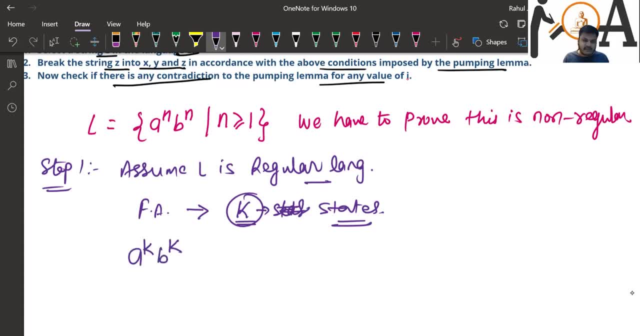 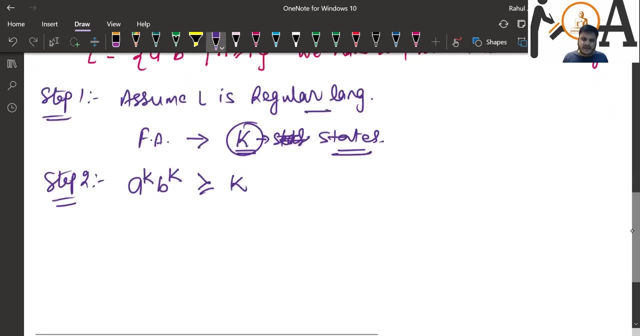 a to the power k and b to the power k is there which should be greater than or equals to k. Step two: how I am saying this? because if there is a finite states are there, then it must satisfy that on completely revolving around that states, on completely revolving. 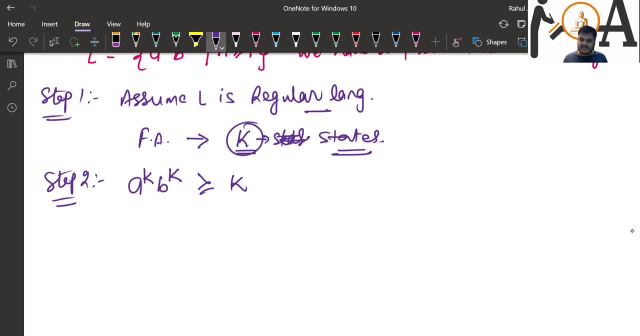 around the finite states. So if there is a finite automata, it must be accepted there. If it is accepted it means that regular, but if it is not accepted it is non regular. However, we cannot prove that any language is regular or not on the basis of that, but only we can prove that it is. 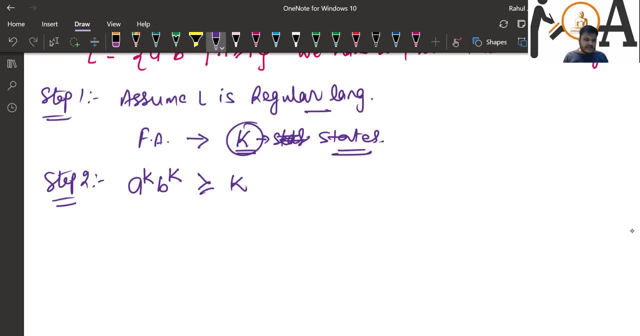 non regular, So I can write it. I can break the string, this w string, into three strings, into three sub strings: x, y and z. Let me break it into the three. So if I break this three substrings, I can break it like, let's say a and in between a, if in between this a is there. 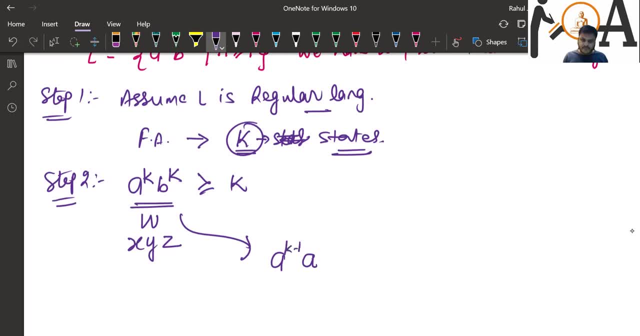 then it is nothing, but it's k minus 1 and it's b to the power k, because k is a certain number of set. Our problem was to prove a to the power n and b to the power n where n is greater than equals to. 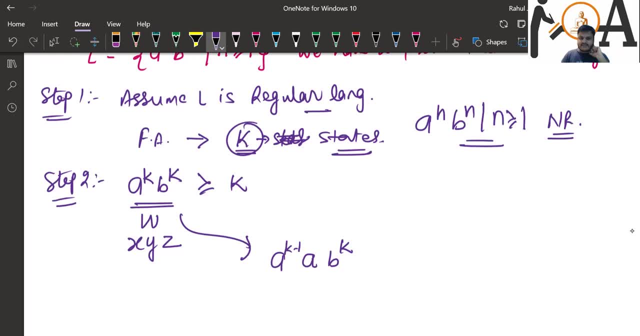 1 as a non-regular correct. So let's say, for particular k states, we are taking the problem and if it is a non-regular, if it is a regular, then it should be followed, it should be accepted with the finite set of states. and I can break this. I can break this problem into this three. 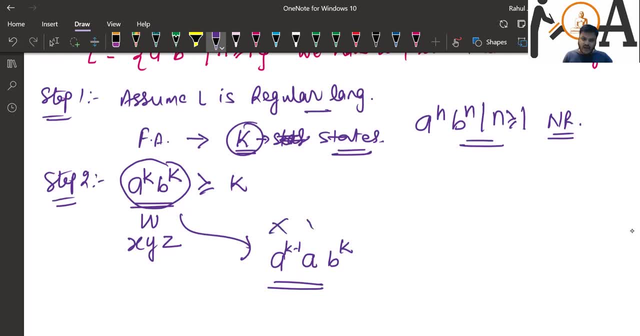 substrings, because if I am taking it x, y and z, y is a, if y is a, then x would be a, k minus 1 to balance. this isn't it. and this b to the power k is z. Okay, now now x into y to the power i and z. it should be followed for. every value of i should be greater. 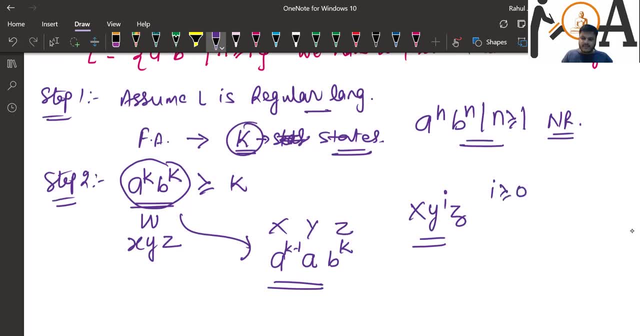 than equals to 0.. Why? Because it follows the principle of Pesonal that if let's say, let's say if a is greater than or equal to 0, then it should be followed, for every value of i should be greater than or equal to 0. 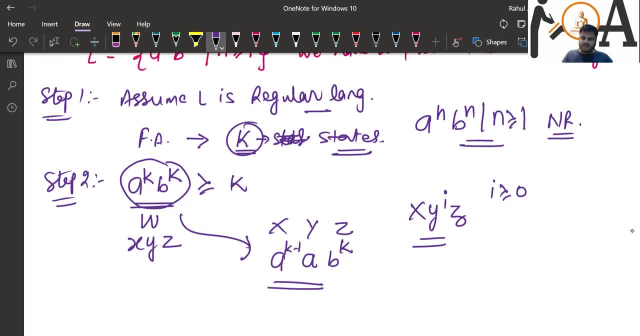 say: value of i is 1. if the value of i is 1, it should be 1. in that case, a to the power k minus 1 into a and b to the power k. it's nothing, but it's a to the power k and b to the power k, which. 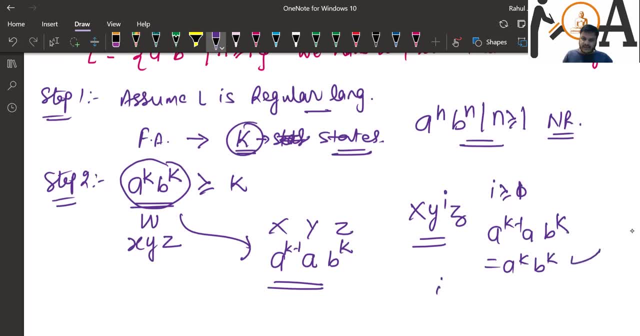 is a part of our language. but what if the value of i is 2? if the value of i is 2, in that case it would become a to the power k minus 1, a square, and b to the power k because y to the power i is. 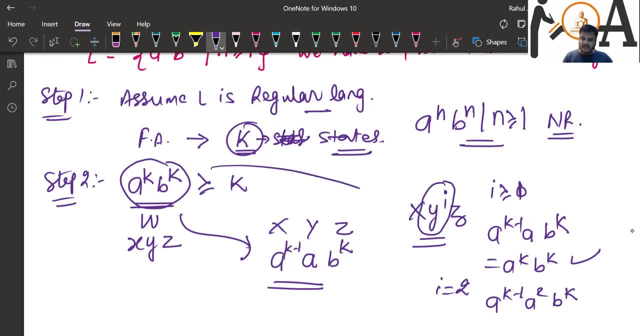 there, i have to, i have to break this string in this format: x into y to the power i and z. if i put i to the value as a, 2 in this case, in this case, what is the resultant string? the resultant string is a to the power k plus 1 and b to the power k. 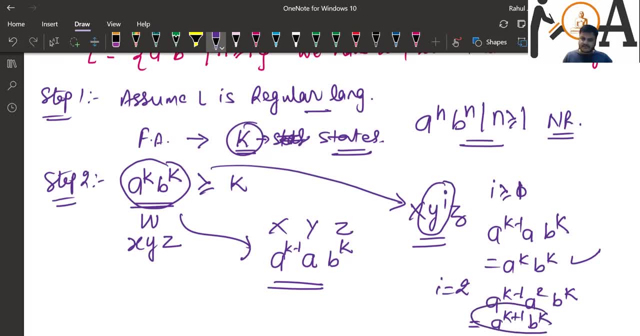 but this string. but this string is not part of my language, isn't it? this string not belongs to my language. thus i can say that it is not following, it is not following pumping lemma. it is not following pumping lemma because if it is following pumping lemma, then on repetition of it, then on. 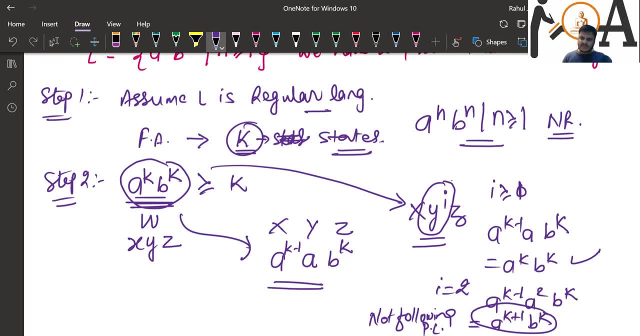 repetition of it on i, many times, many times. it must be accepted somewhere, because if it is a finite length string or it may be some kind of infinite length of a string, and if it is a regular, if it is a regular it means that somewhere cycle may be, exist or somewhere. 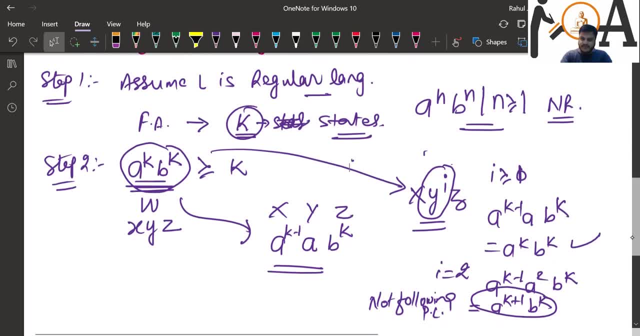 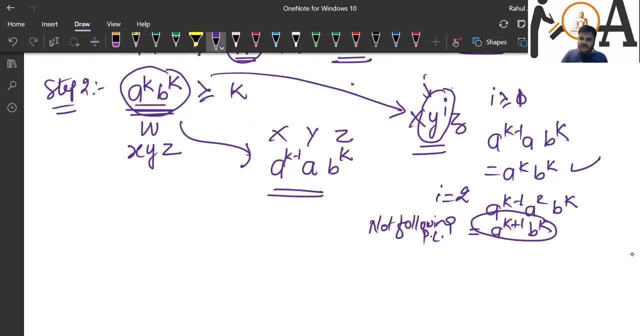 loop may be exist and with the help of the loop or with the help of cycle it would repeat and will be accepted. but here you can simply see that if i can increase the value of i as a 2 or 3 or 4, that is more than one in the case, my resultant 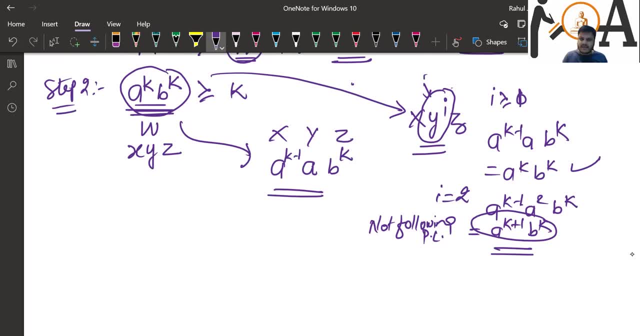 string will become like this, which is not the part of my language, because my language is a to the power and b to the power, and n should be greater than equals to one. it means that a and b should be equal, but here a and b are not equal because pumping lemma says that i have to take a string. 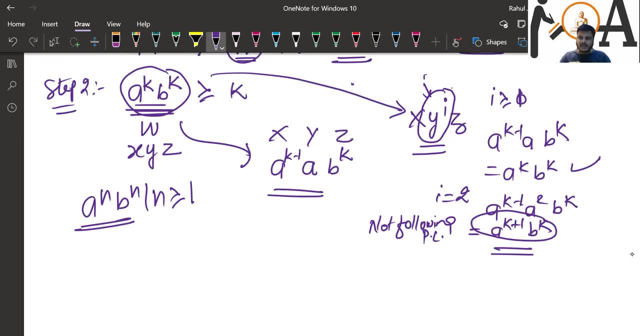 string length, just one one greater than the number of the stats. If my finite automata is having n stats, then the pumping length should be n plus one, So that I can say that if any string of n plus one length is accepted by this finite automata, 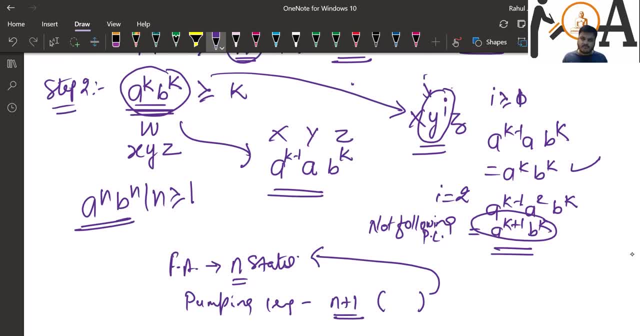 it must have at least one cycle or loop. Thereafter we can say that it would be accepted by finite automata, because if I am taking n plus one length string and my finite automata is having only n stats, in that case how this string is going to be accepted? 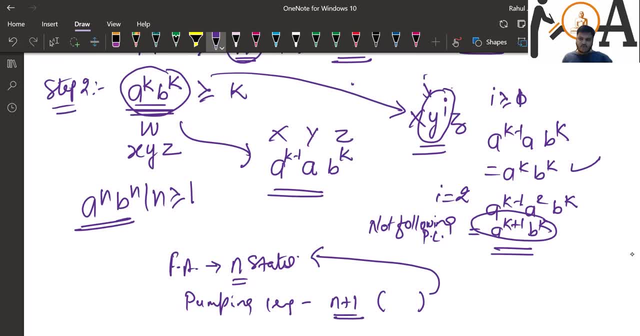 on the final state. I must have any cycle or any loop. They're only possible now. This is the concept of. this is the concept of Pisan-Hall principle. This is the concept of Pisan-Hall principle, isn't it? 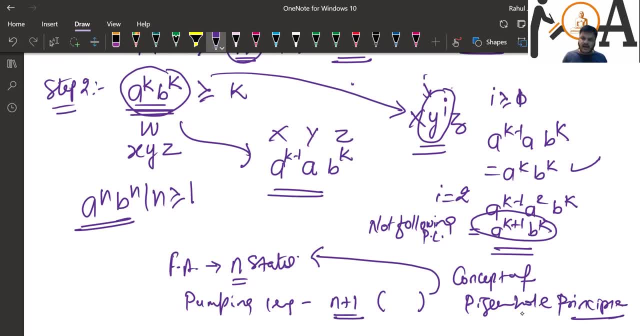 Using that, we can simply say that if we are going to increase the value of i, but the resultant string is not part of our string, Hence this string is not possible. It means that it is not following pumping lemma. So if it is not pumping following the pumping lemma, 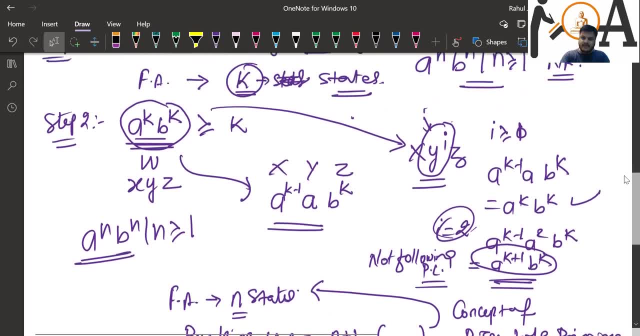 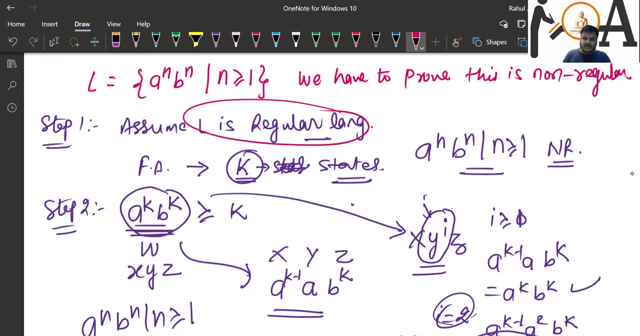 it means that it contradicts our assumption. It contradicts our assumption. What was our assumption? That L is a regular language. but it contradicts because it fails to provide that it's having a pumping lemma. That's why we can say that this is a non-regular language. 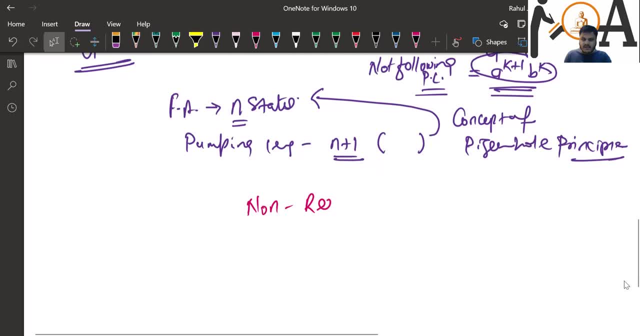 This is a non-regular language because it failed to aspire all the properties of pumping lemma. So this is all about pumping lemma. I hope the concept is very much clear to you. Further, if you are having any kind of doubt or confusion, 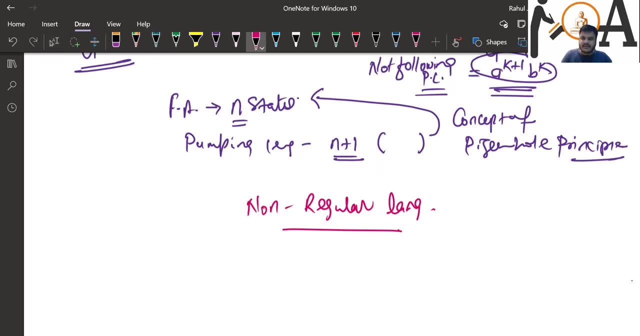 you can ask me. Thank you so much. Have a very nice day. Jai Hind, Jai Bharat.